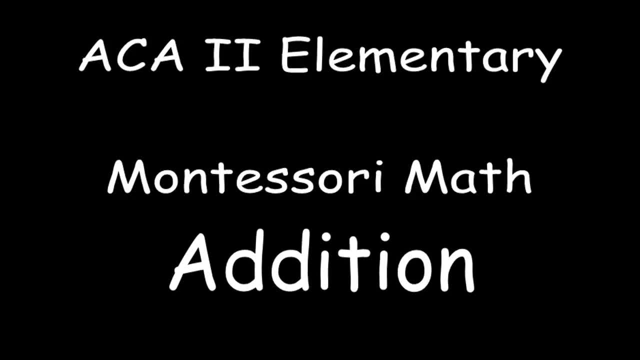 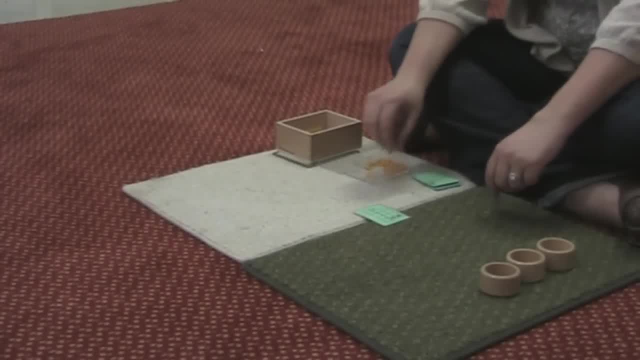 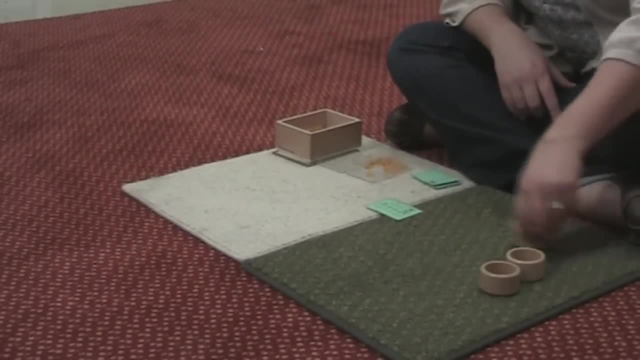 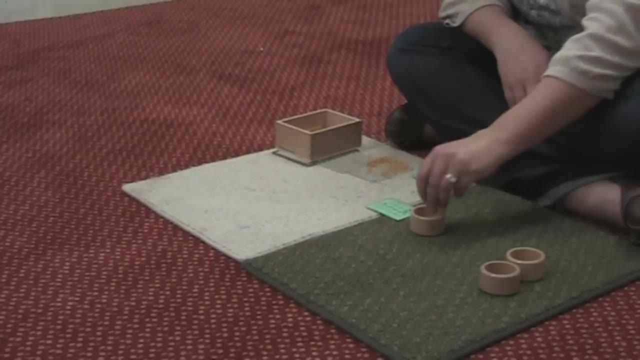 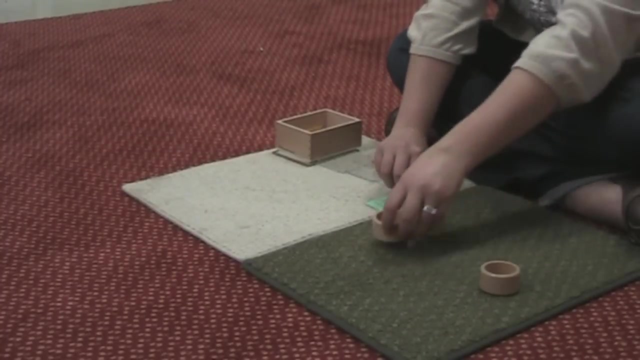 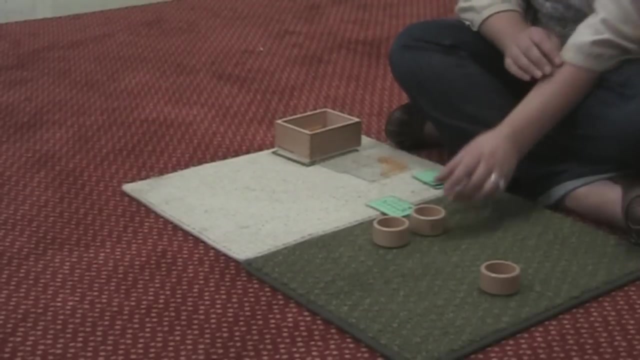 We're going to be doing SA, static addition, So we'll start by building our top number of our units, which is six- One, two, three, four, five, six- And then we will add our second units and another cup of two units- One, two- So now we have our six units on. 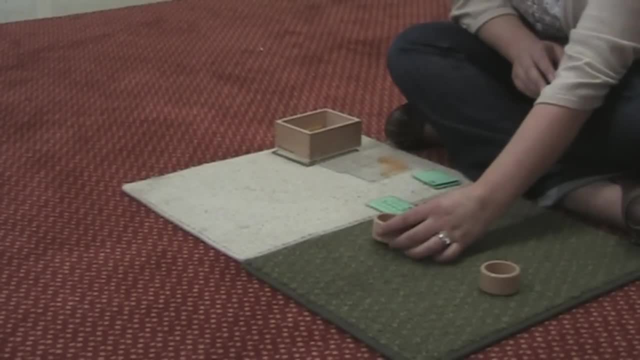 top And then our two units on the bottom, And we'll take our two units and we'll add them to our six units And then we will count them up into our cup. One, two, three, four, five, six, seven, eight. So our answer would be eight. 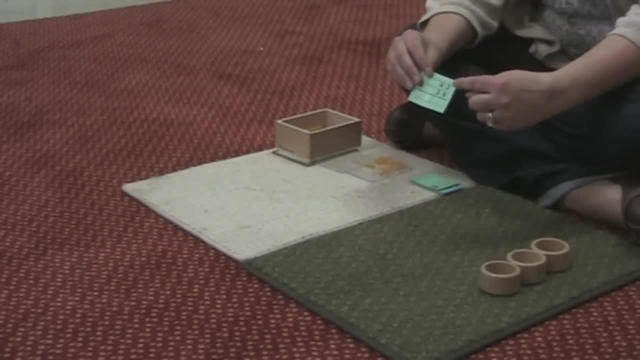 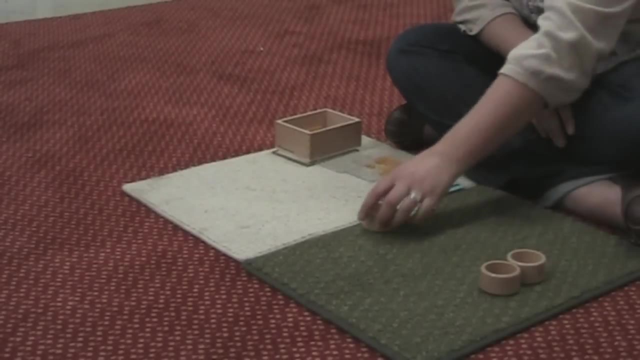 So now we'll do double digits, Double digit SA. So we have units and tens And we always start with our units. So we'll start by building our units on the top, which is three, One, two, three, And then we'll. 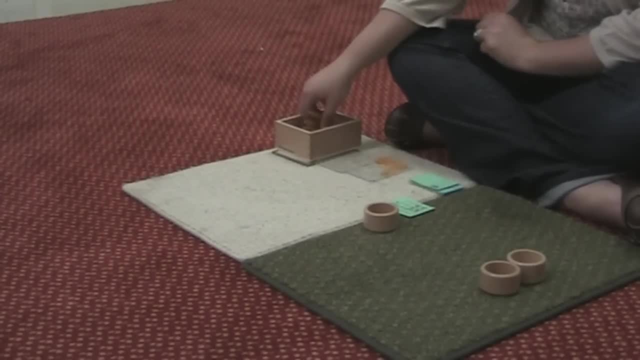 build our tens, which is six, ten, twenty, thirty, forty, sixty, seventy, And then we'll build our top Writing out our units. on the top says: go to your roll, 물론. the top. Then what we're going to do is we're going. 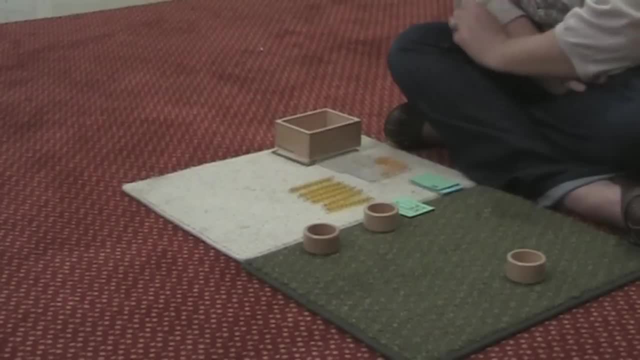 to rebuild our top. So four times the six units. Now let's do one rule. So we're going to do two units. We're going to include the top number, the middle number, the bottom number, the middle number and the감 thousand plus AND plus filled. 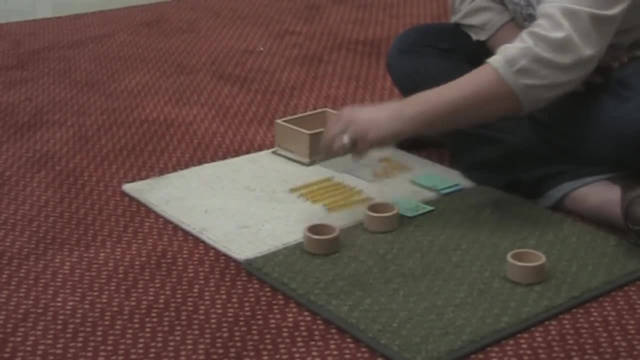 with distance. If we have two top figures on left and we have 18,, 20,, 21,, 22?, it's going for six, And then we have four top figures at bottom. So getting the bottom number out first. 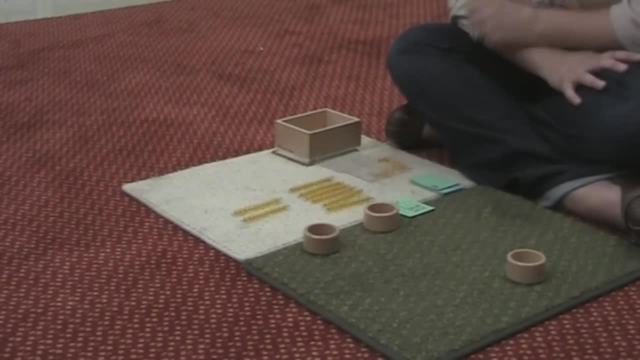 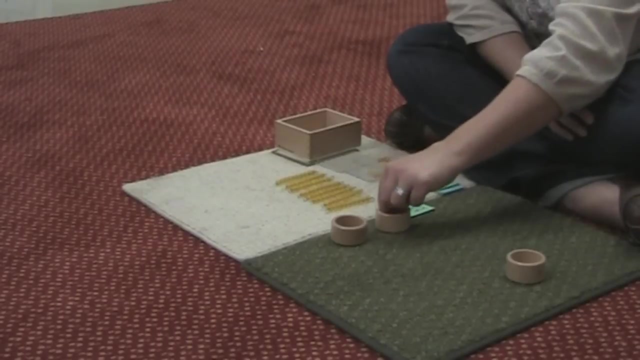 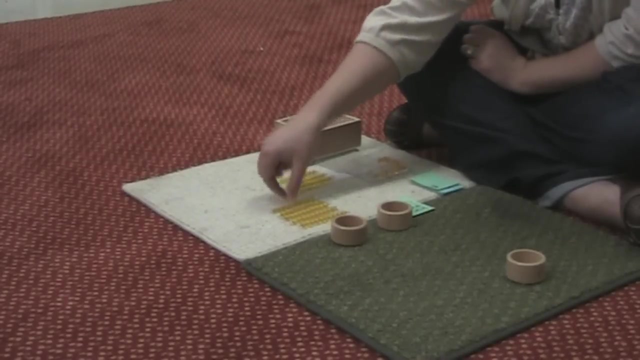 40, 60.. number 10, 20.. Once we have our top number 63 built and our bottom number 26 built, we will add them together, push them together and then we'll count, starting with our units 1, 2, 3, 4, 5, 6, 7, 8, 9.. We have 9 units and 10, 20,, 30,, 40,, 50,, 60,, 70,. 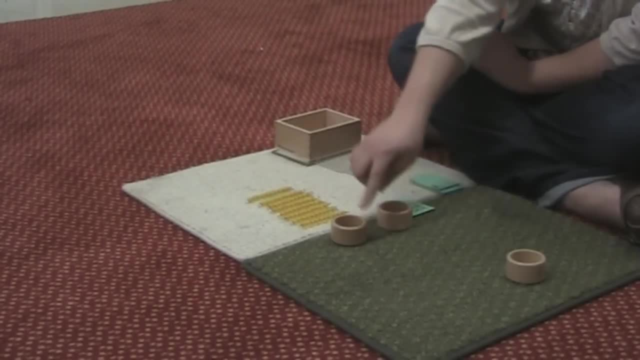 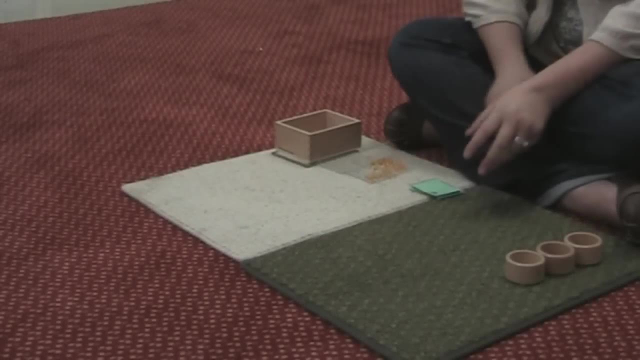 80. So our answer is 80. Now we're going to go to DA, also known as Dynamic Edition. We're going to do 25 plus 7. And with DA as well, just like every other, we always start with our units, So we'll get. 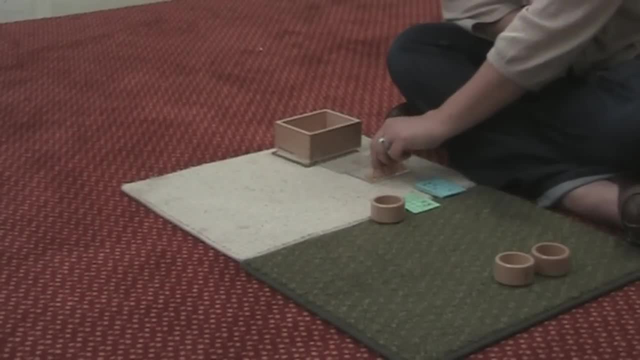 a cup for our top units And we'll put our 5 units in the cup: 1, 2,, 3, 4,, 5,, 6,, 7,, 8,, 9, 10.. 1,, 2,, 3,, 4,, 5, 6,, 7,, 8,, 9, 10.. 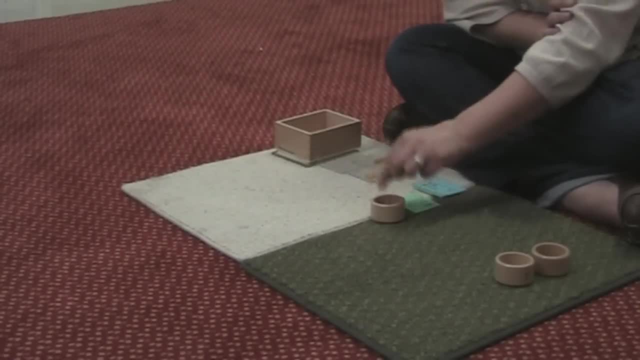 1,, 2,, 3,, 4,, 5.. And then we'll build our 10s, which is 2.. So 10, 20.. We have our top number built, 25.. Now we're going to build our bottom number, which is 7 units. on the bottom, 1,. 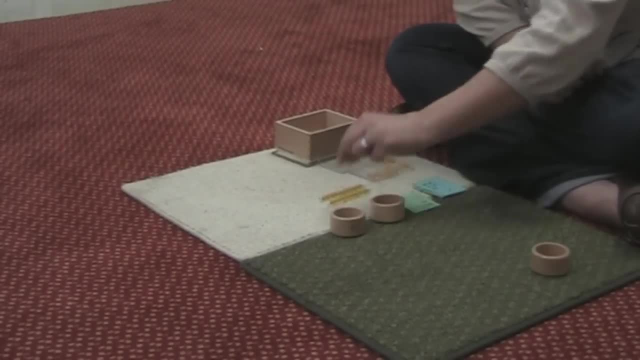 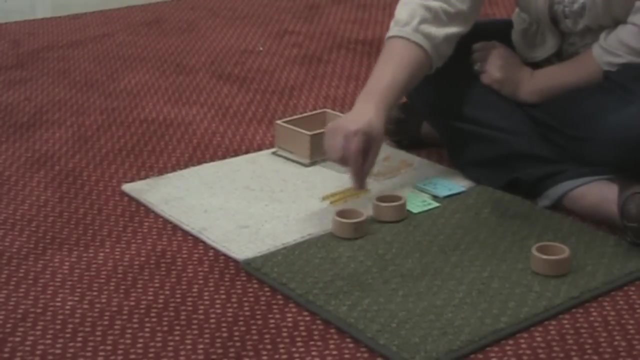 2,, 3,, 4,, 5,, 6,, 7,, 8. 7.. Now we have our top number built, 25, and our bottom number 7.. And we're going to add them together. And now we're going to count: 1,, 2,, 3,, 4,, 5,, 6,, 7,, 8,, 9,, 10.. And when you 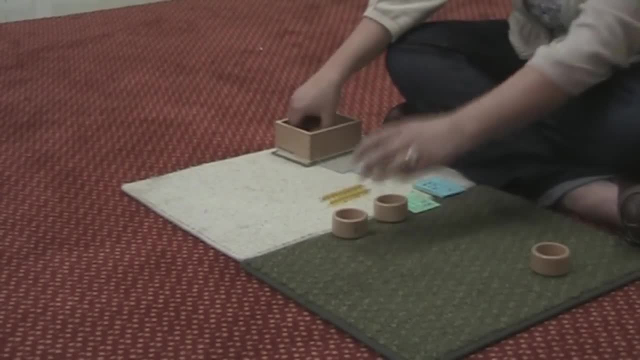 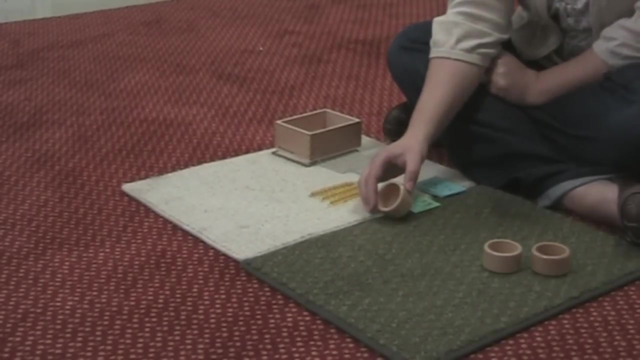 get to 10, you're going to trade in your 10 units for a total of 10 units And then you're going to trade 10 bar. So you would take your 10 units and you would trade them in and you would get your 10 bar and put it out. So now you have 2 units and 10,, 20,, 30,, 10s. 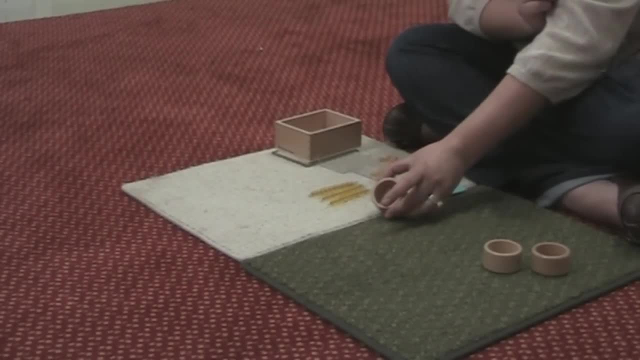 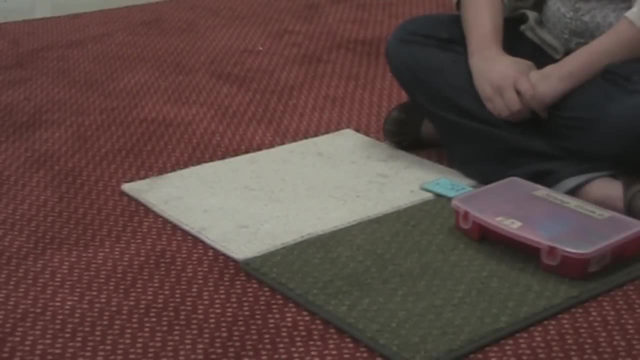 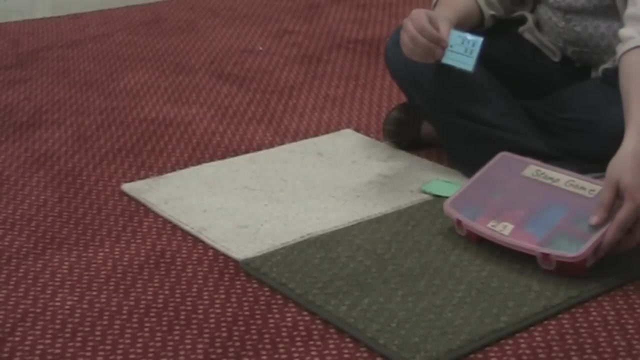 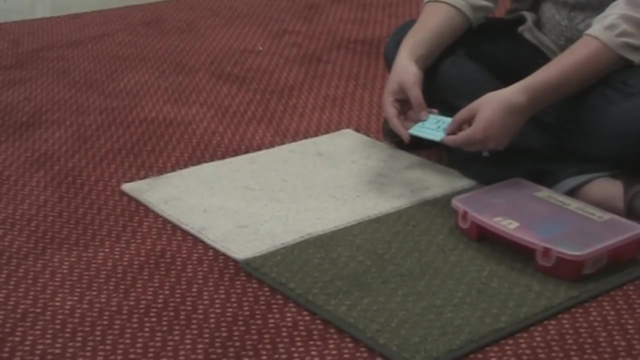 So your answer would be 10,, 20,, 30,, 2.. So now we're going to do dynamic addition: 1,, 2,, 3,, 4,, 5,, 6,, 7,, 8,, 9,, 10,, 11,, 12,, 13,, 14,, 15,, 16,, 17,, 18,, 19,, 20,, 21,, 22,, 23,, 24,, 25,. 26,, 27,, 28,, 29,, 30,, 31,, 32,, 33,, 34,, 35,, 36,, 37,, 38,, 39,, 40,, 41,, 42,, 43,, 44,, 45,, 46,, 47,. 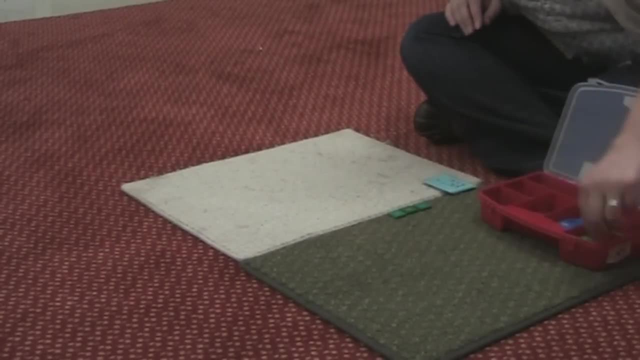 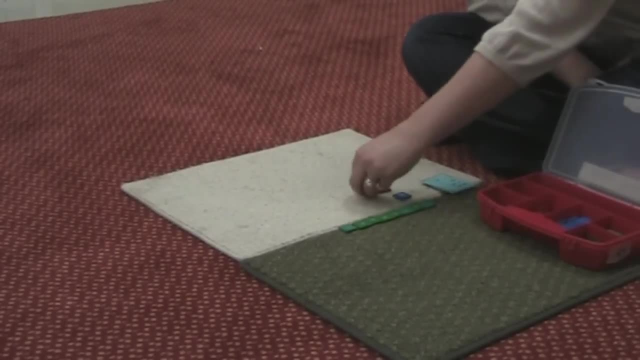 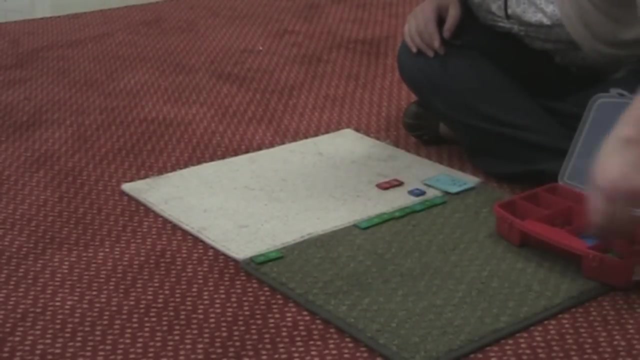 Now that I have my top number built, I will begin to build my bottom number: 1,, 2,, 3,, 4, 5, making sure there's enough space so you can see the difference. Now I'll build my bottom.